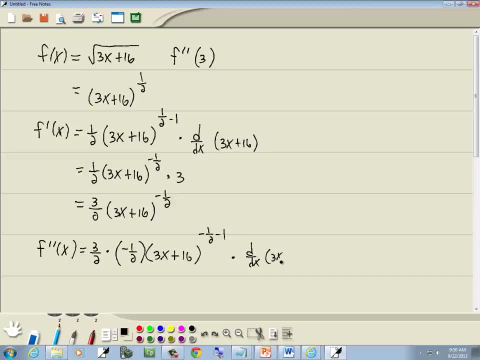 And then again times the derivative of what's inside your parentheses. Keep in mind what we're trying to find, Because I'm getting ready to scroll. We're trying to evaluate that. So after we find the second derivative, we want to plug 3 in for x. 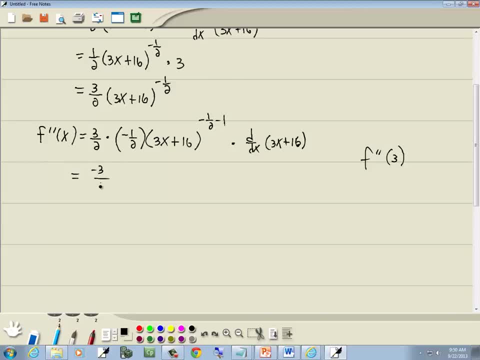 Okay, 3 times negative: 1 is negative, 3.. 2 times 2 is 4.. 3x plus 16.. Negative: 1 half minus 1 is negative: 3 halves. The derivative of 3x plus 16 is 3.. 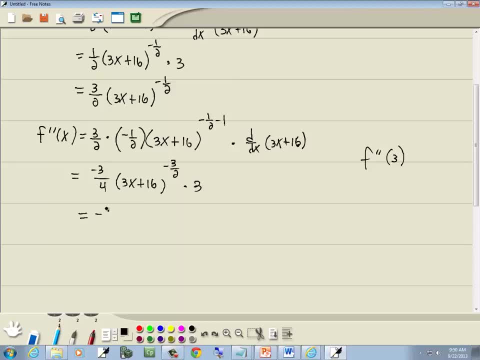 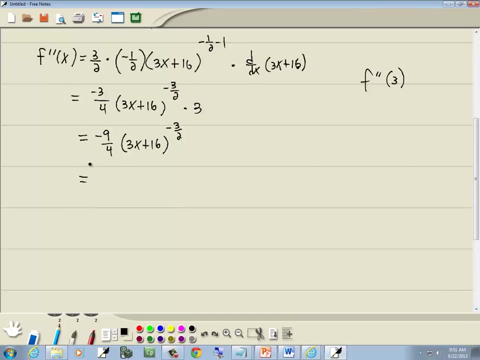 So then 3 goes out in front. So that gives us negative 9 fourths, 3x plus 16. to the negative 3 halves. We don't want any negative exponents, So the part of the negative exponent I'm going to take to the denominator. 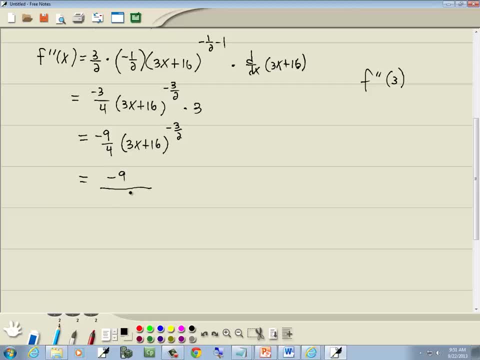 So this is going to become negative 9 over 4 times 3x plus 16 to the positive 3 halves power. Remember you take anything opposite in a fraction and assign it to the exponent changes. So the negative 3 halves becomes the positive 3 halves. 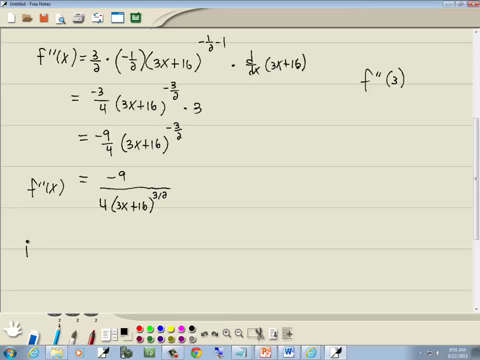 And that's our second derivative. Well, we now want to Plug in 3 for the x, So everything remains the same. I'm going to make these brackets just so I can separate them. And where our x was, we put in parentheses. 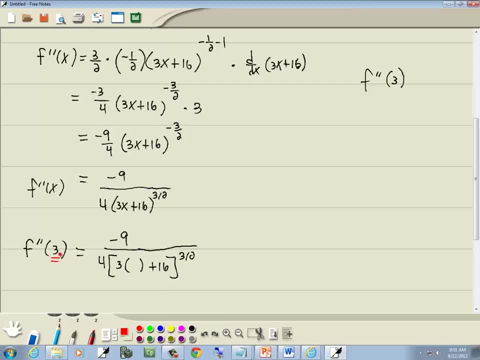 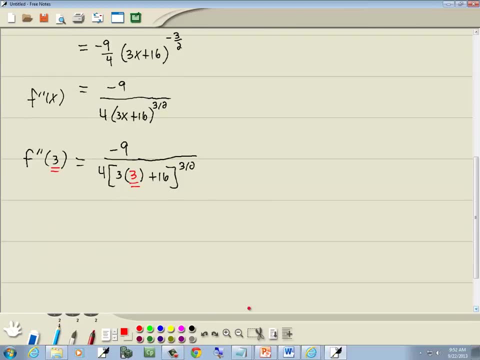 And again, evaluating a function is: whatever number is inside your parentheses. here is automatically what you put in right here. So we put a 3 in there. So that gives us negative 9 over 4.. 3 times 3 is 9 plus 16. to the 3 halves power. 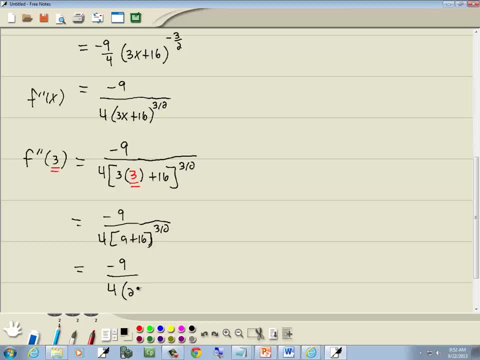 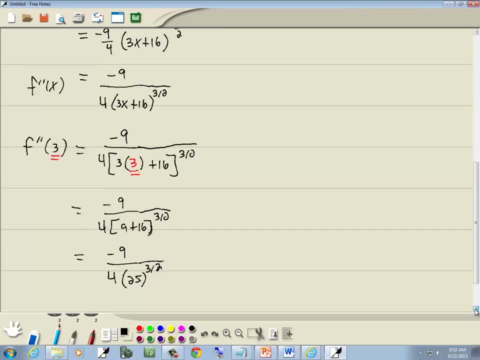 Which gives us 4 times 25 to the 3 halves power. Now we had a property back in intermediate algebra, algebra 2.. It said: if you have a number. It said if you have a number. It said if you have a number.